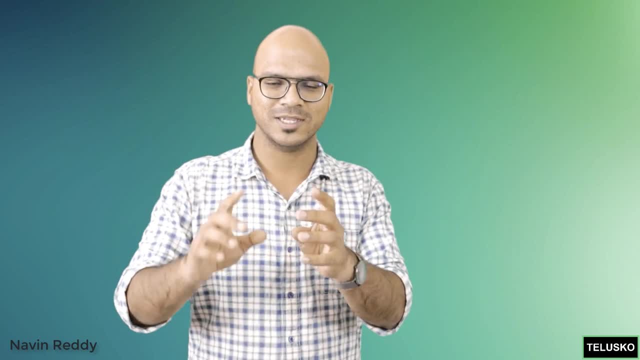 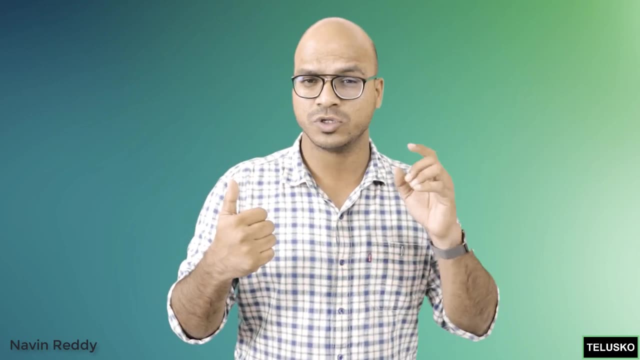 if client wants two plus two should be five, then you have to write a software which says two plus two is five. Maybe there's one which is interest right. So you have to match the client requirement. So when you build a software the software should work and it should work efficiently and correctly. 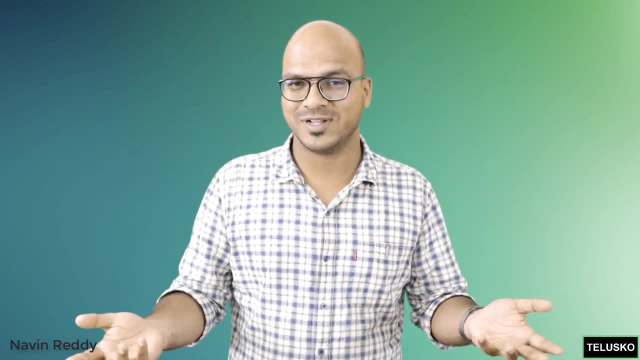 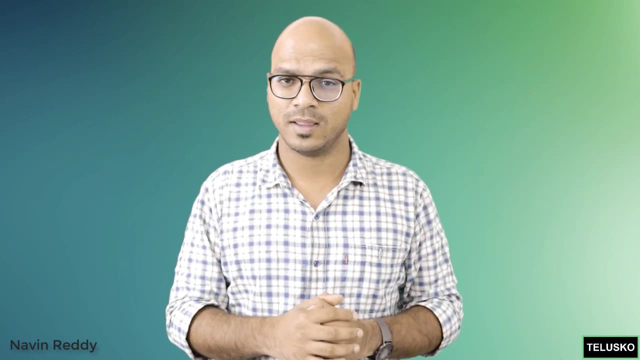 But then at the moment you said testing- you know a lot of people. they don't like this word as well- testing- Why you have to test. We love development, but testing is important. In fact, we have a video on that as well- The moment you said testing, we have two words. We have two words. We have two. 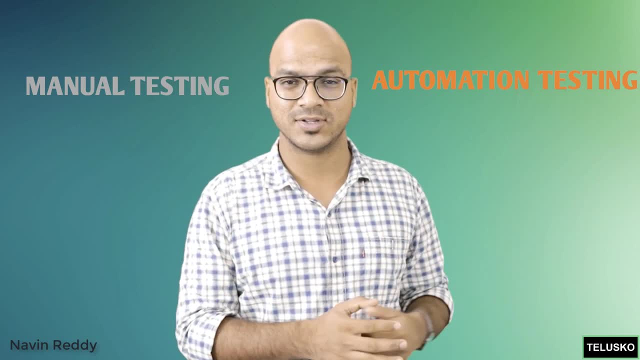 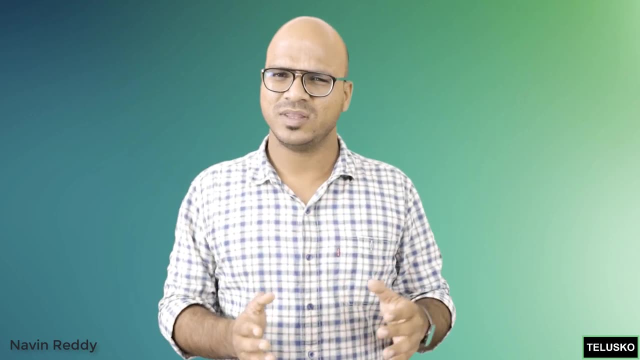 types there. One is manual testing and second is automation testing. So manual simply means you are, you're testing everything manually, So you are checking the outputs, You are giving some input. On the other hand, we have automation, So basically you write script to automate your testing. 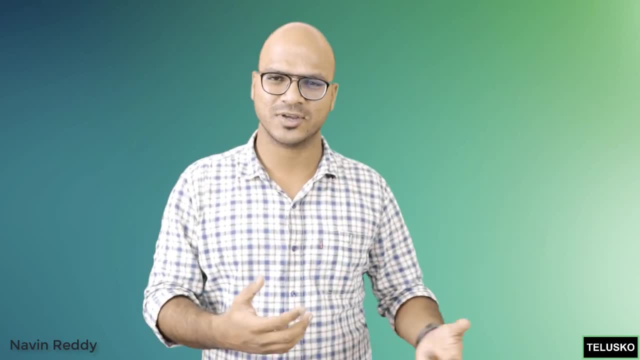 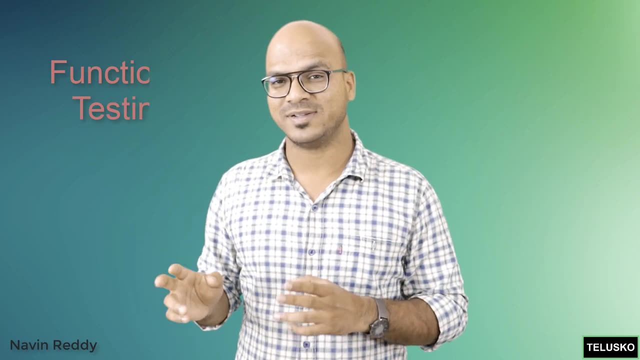 One of the way you can do that in java is using junit, So you can write junit test cases. In different languages we have different way of testing it. So basically we have one more classification of testing, which is functional testing and non-functional testing. So basically, 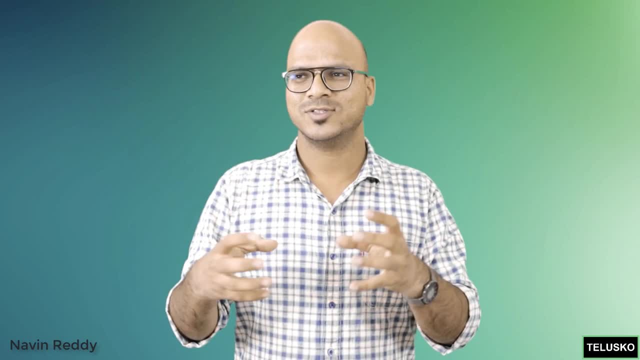 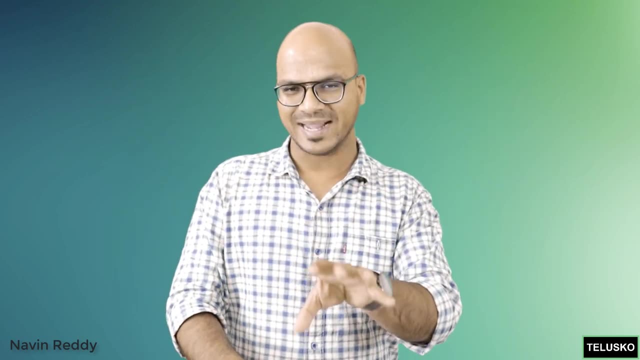 when you say functional, it simply means you are testing the code. So let's say, if you write multiple classes, multiple methods, you are testing them. So you're basically testing the actual working on the software, right? That's the functional testing: the code part and then input parts. 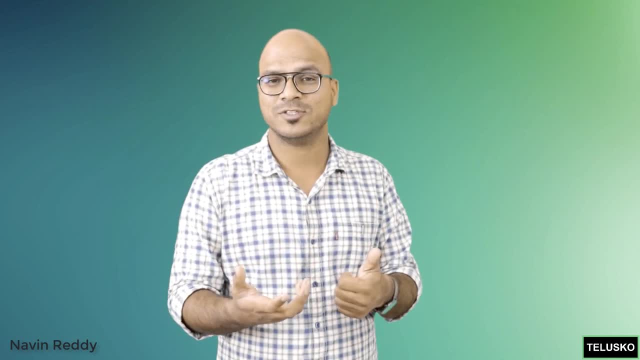 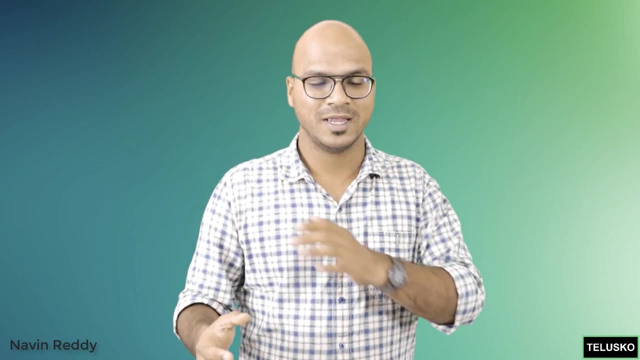 But what about the performance? What about the scalability? So, example: when you say performance, when you, when you run the software, it should work smoothly, right, It should. example, if the softwares which we use for editing purpose, they should not give any lag, right, When you play a. 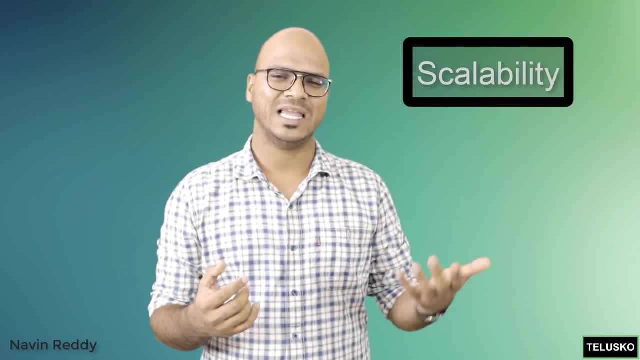 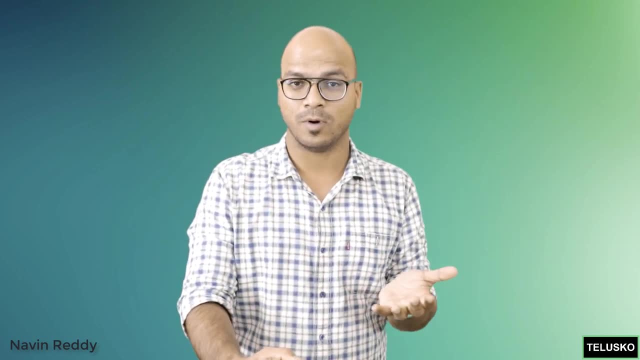 game. it should be, it should give proper performance. So when you say performance, it should give proper performance. So next one is scalability. So let's say: can you, can you scale your application? So let's say: if you deploy an application on cloud, can you scale it? That's also important, right? So 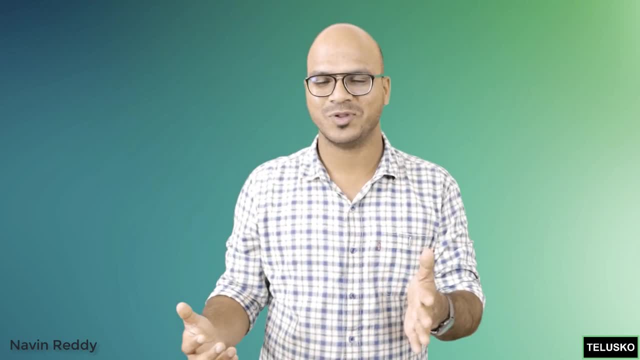 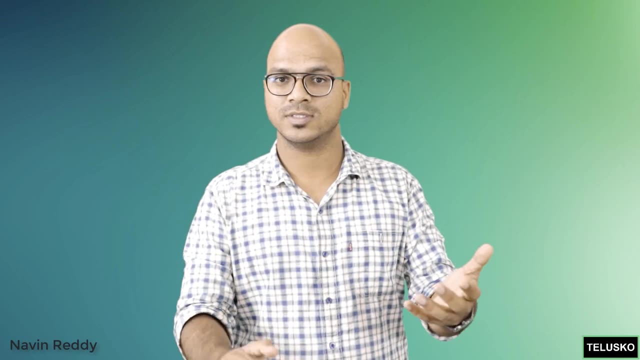 don't just build a software which cannot scale but it works. No one's. no one's want that right. So your software should be scalable. So those things comes under non-functional. Also about load balancing or loads Can your software? takes load Example. let's say software for hotstar and recently. 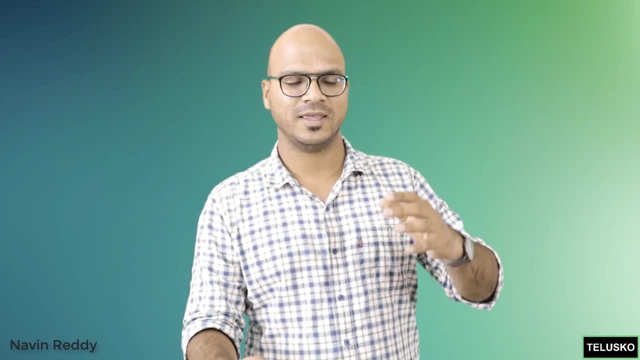 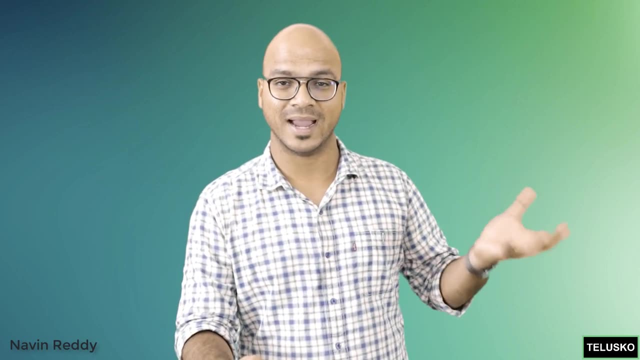 we had india news and match, which is the same final, and then at one point there were two, 25 million users watching at the same time. So can your hand, can your software handle that load? So that's also important. So that comes under non-functional. So how do we test it? So basically, 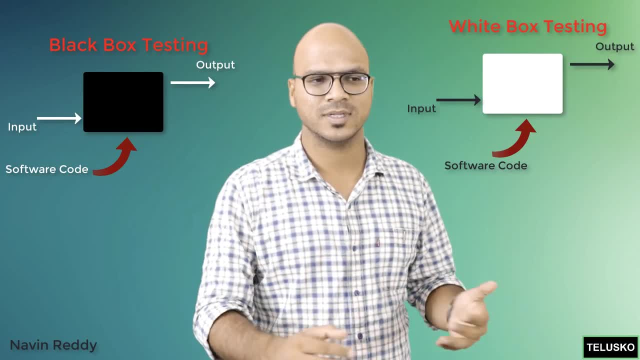 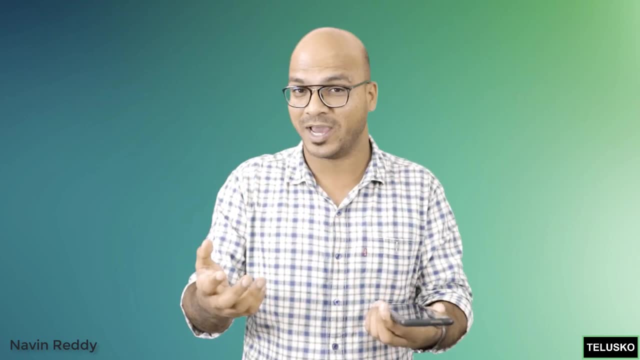 we have two techniques. One is black box and second is white box. Now, this black box, you can imagine if you want to test a mobile phone. Now you don't know how, how this phone works internally, So what you will do. So when you buy a new phone, or when you go to a showroom to buy a new phone, what you 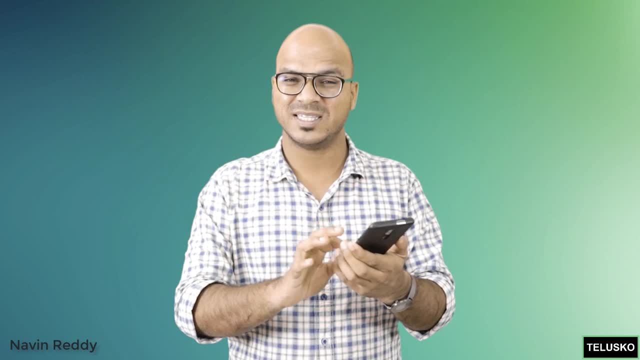 do you unlock the phone? you check: Okay, so unlocking works. You want to test the cameras. you know, open the front camera So it should come out, So you can see that the phone is working. So you can see that the phone is working, So that works, That's great. So you then you test the battery by 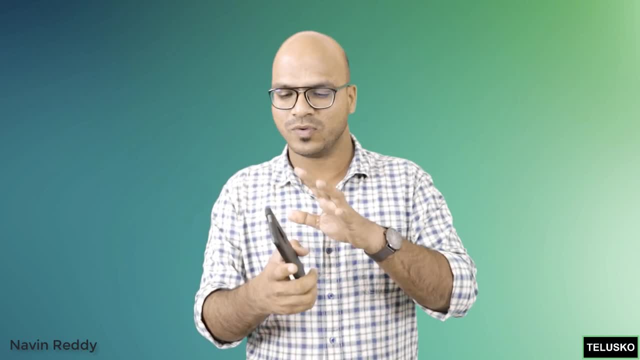 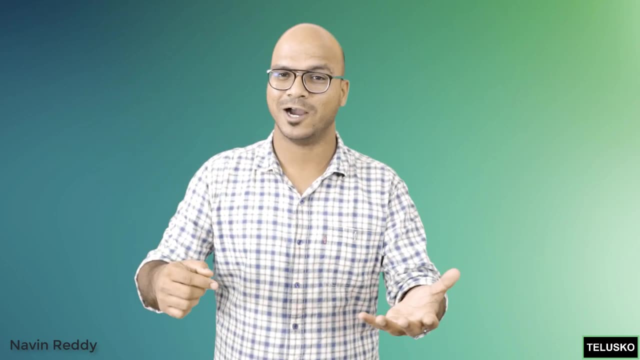 how you test the battery doesn't matter. So you will test the screen, everything right. So you will test the phone outside, right? You don't know how it is, what is going on inside, and that's, that is black box. You give the input, you expect the output. On the other hand, we have white box testing. So 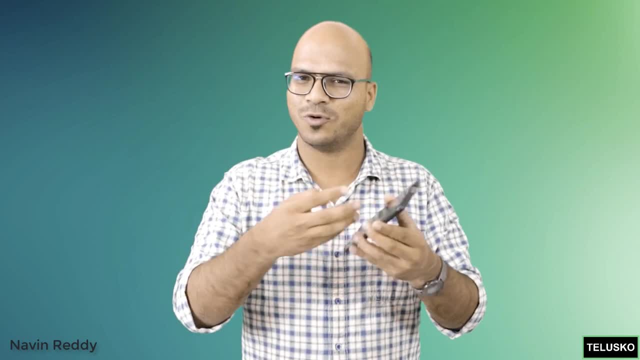 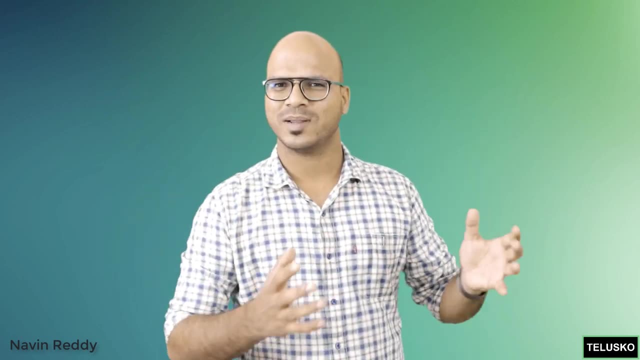 you don't just test the outer working of the software, but internally. So you will open this and you will check each and every component how that works. That is white box, So in coding terms, you will check the actual code. Okay, so we have talked about types of testing and techniques. So 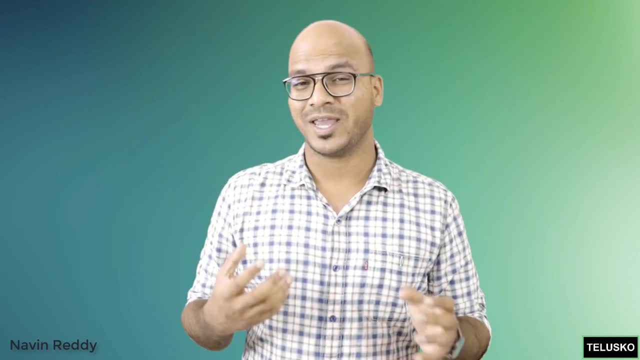 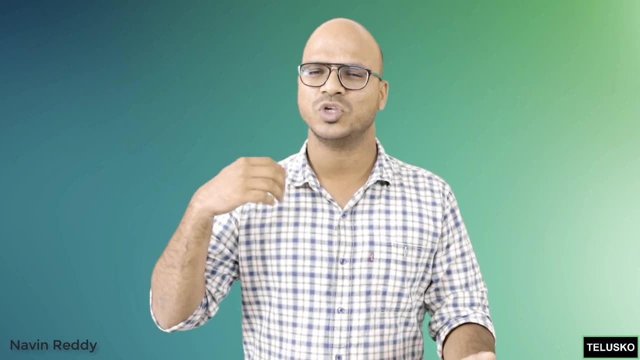 different levels of testing. So let's stick to Java here. In Java we write a lot of classes, right? So we have classes and each class will have certain methods. So now you want to test the smallest part of your software which is a class. So you will test a class and we will call them as. units. So basically, you will test each class which is units and we will call them as unit testing and in Java, if you want to achieve that, we have JUnit- Then once you test each and every component now, you will combine all the components to test this as a software which is integration testing. So 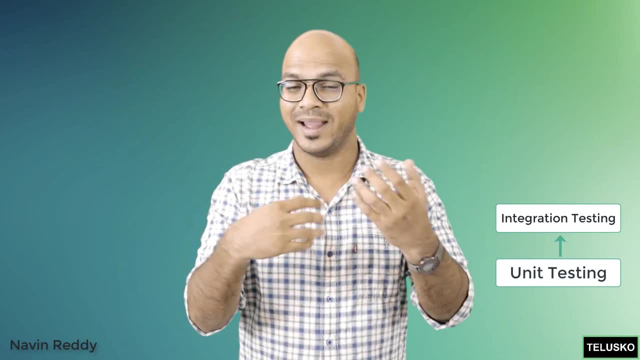 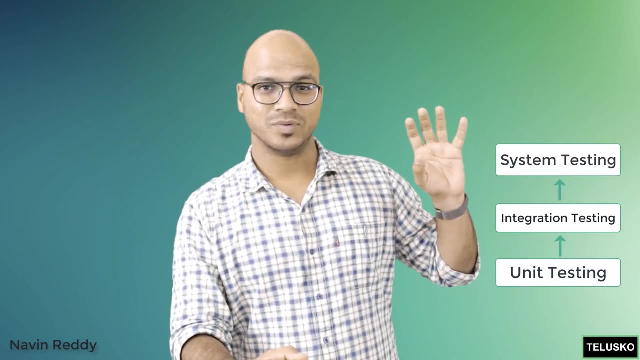 you will combine a lot of different classes and then APIs, And now, once you have that you will, you will do system testing. It's the overall testing of your system if you deploy it, How that works with other softwares, or about the and with the actual data. Now, once you have your, 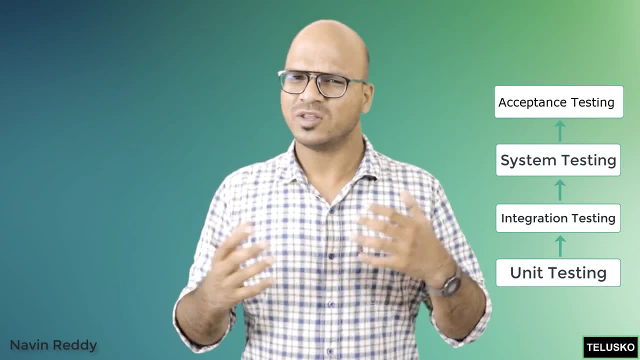 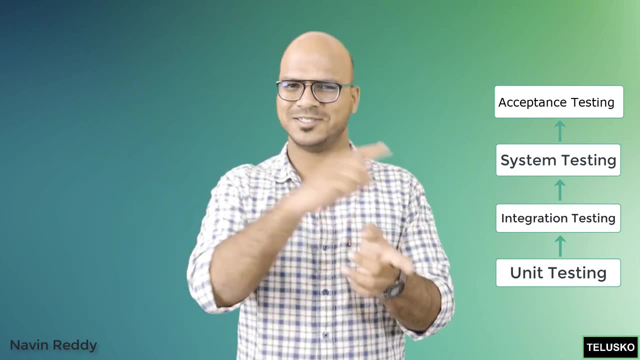 system testing. next step we'll go for is acceptance testing. Now, this is where you will try to match your software with the user requirement. right, So you will. you will have the business requirement with you and you will try to match: Hey, is it matching? Is it matching? If that matches, that's. 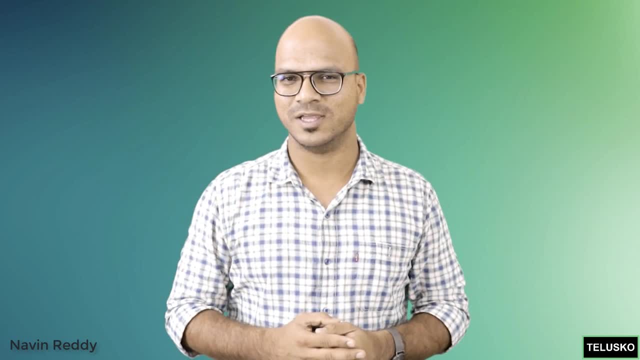 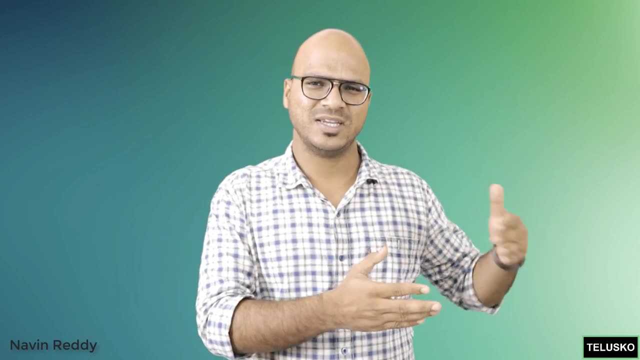 fine, And then, once you have that, you will go for acceptance test. So, basically, we have these four levels available And then to do this, to do the actual testing, we have different type of people, right? For example, when you are a developer, we normally focus on the unit testing and integration. 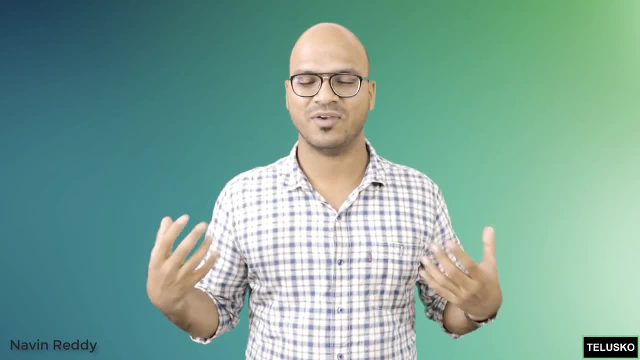 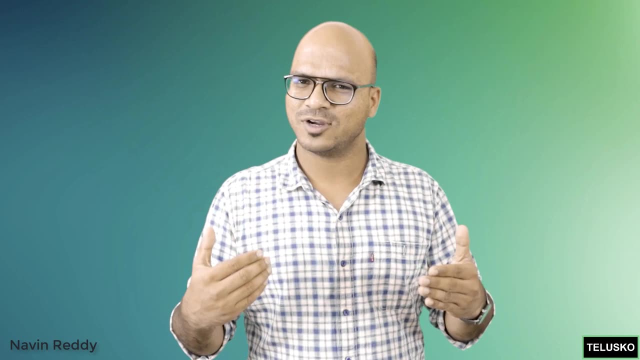 as well. So nowadays things are changing. Initially we used to have two different groups, but now we have an agile team where everyone does everything. So, as a developer, it's your responsibility at least to do the first part, which is unit testing, Because when you write a class, you have to make sure that.